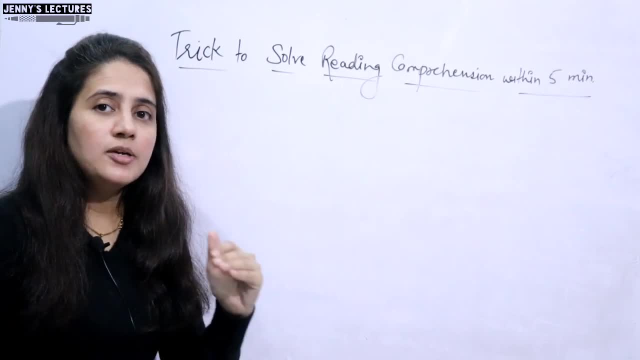 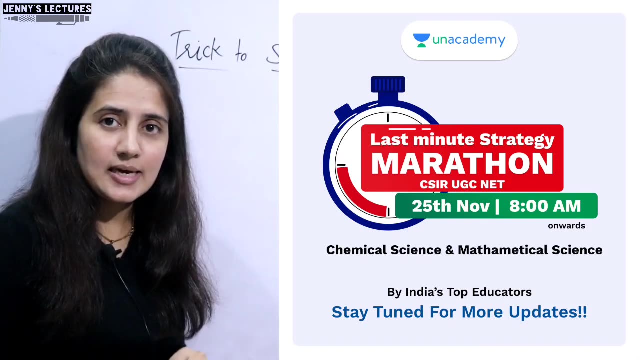 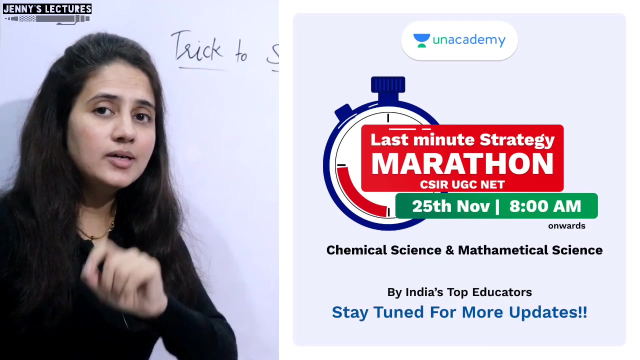 after the exam. But you can boost your preparation with the last minute strategy marathon at an academy for the subject chemical and mathematical science. It is going to be held on 25th of November. In these classes they are going to discuss some last minute tips that are going to be 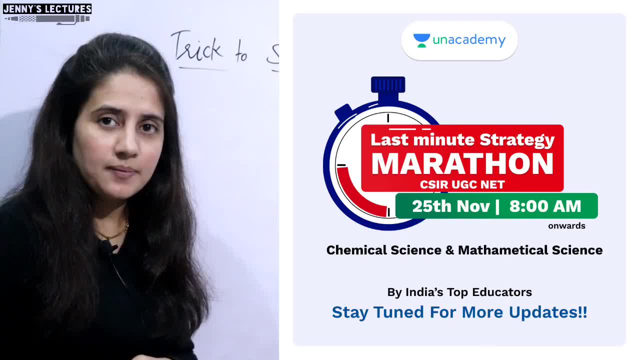 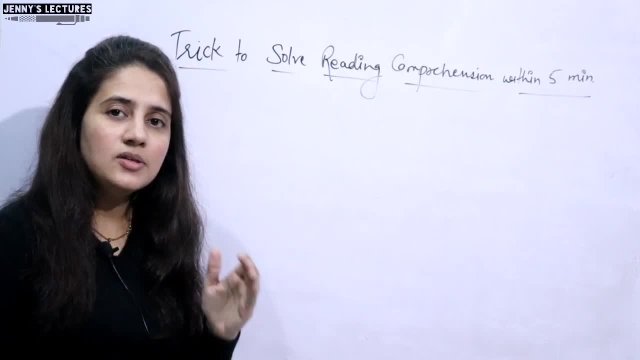 very helpful for you guys on your exam day. And these classes will be conducted by the top educators at an academy And you can attend the exam on the exam day. So you can attend the exam and these classes freely. You don't need to pay anything to take to attend these classes In. 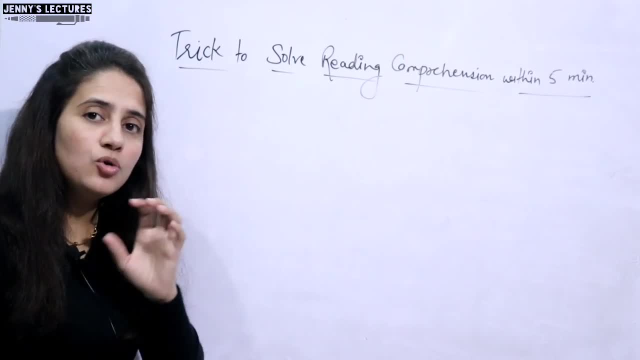 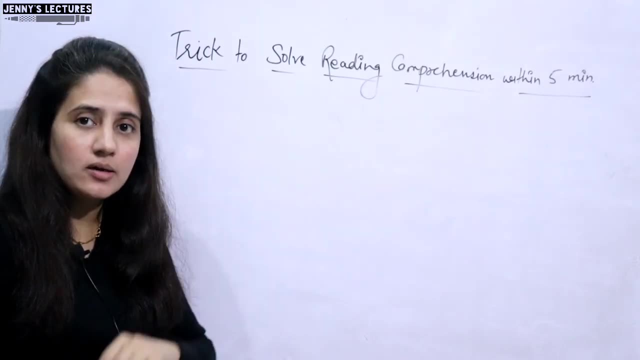 these sessions they are going to discuss some tips about how to stay motivated throughout the exam. Paper strategy, paper attempting strategy from all India rankers. How you can avoid negative marking in your exam because in CSIR UGC net you have negative marking. Tips and tricks to 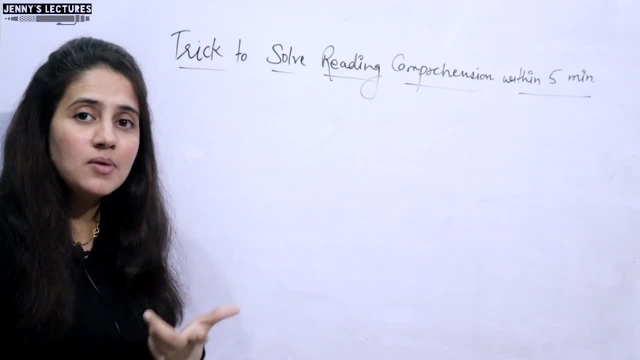 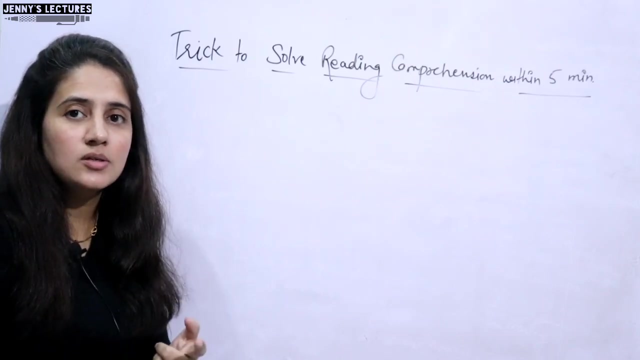 solve general aptitude questions, A smart approach to maximize your marks, Mistakes to avoid while attempting the question paper And how to utilize your three hours timing in a best way for CSIR UGC net exam- These kind of things they are going to discuss. 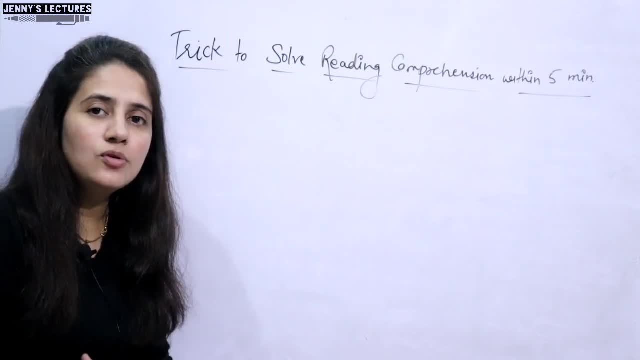 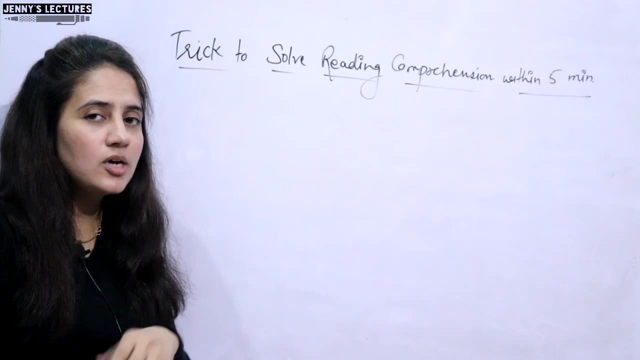 in these classes And these tips would be really helpful for you on your exam day. You don't need to pay anything for that. You just have to do what. to attend these live classes, You just have to enroll All the details and the enrollment link I'll provide you in the description box of this. 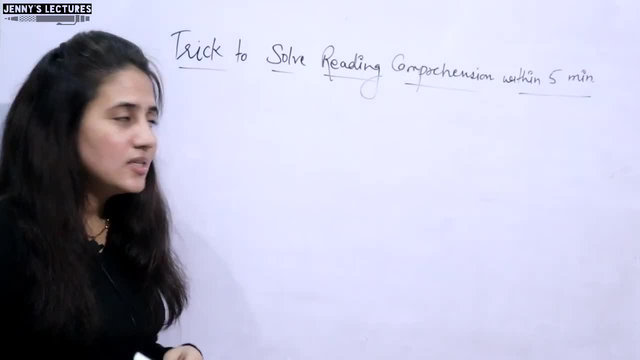 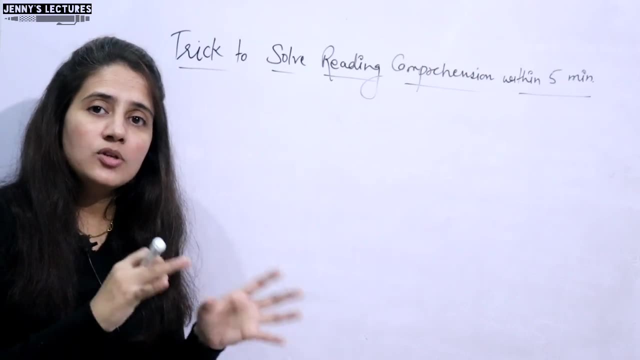 video. If you are interested in learning more about CSIR UGC net exam, please do subscribe to CSIR UGC net exam. You can go and check out Now. let us discuss the trick to solve reading comprehension question within five minutes. See, some students also have this doubt. 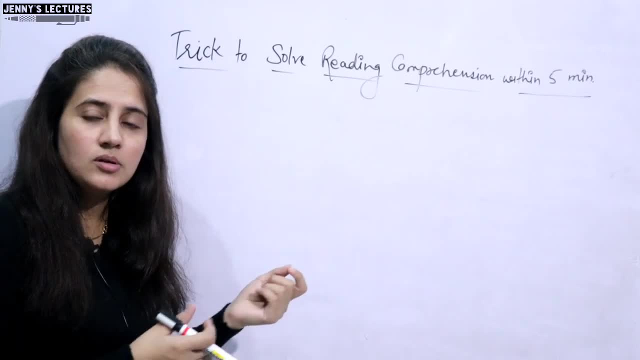 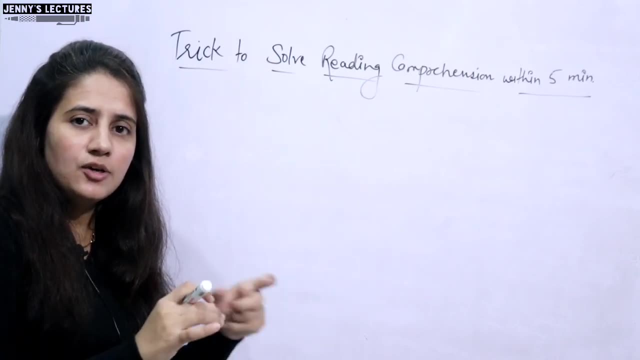 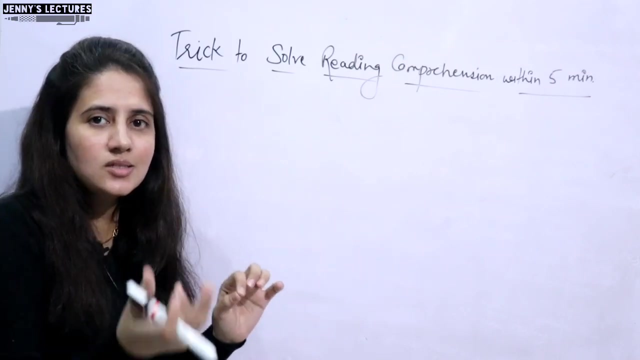 also ask this question that should we solve RC question in the beginning or at the end. So I would suggest neither in beginning nor at end, because if you solve these questions at the end, definitely you will have less time at the end. You have 50 questions and 60 minutes, right And 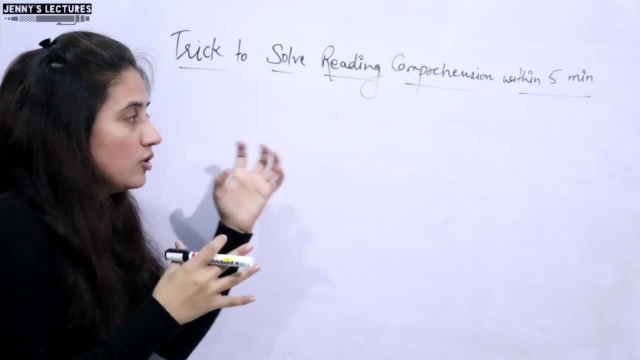 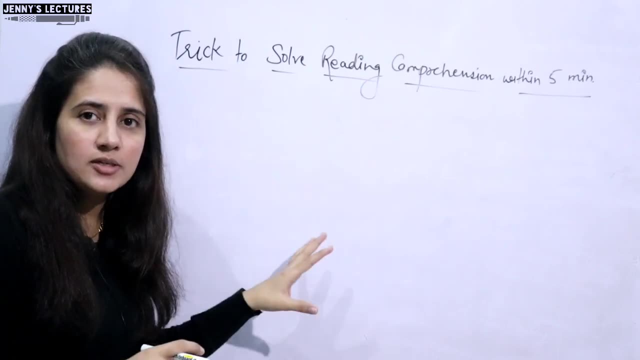 at that time you have less time and you have pressure of solving the question. You have pressure of reading the passage, then solving five questions. Definitely you will not get anything from that passage. if you read that passage, you know in pressure. So if you want to solve reading 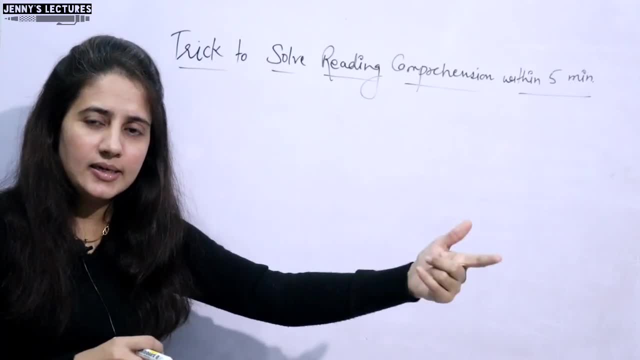 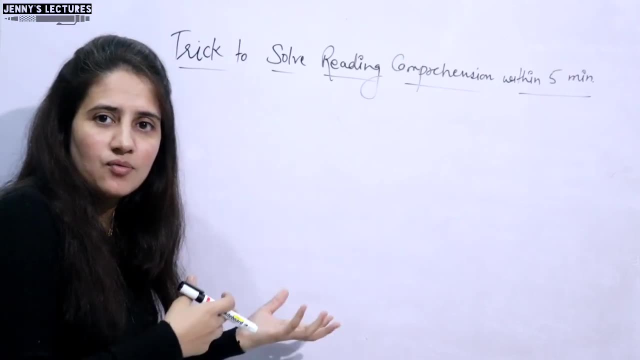 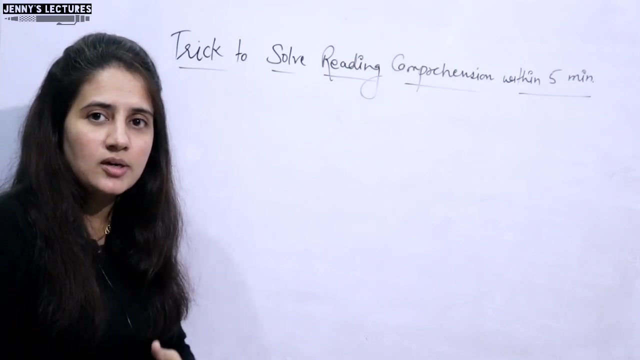 comprehension question. do not leave it for the end and do not solve these questions at the beginning, because sometimes, yeah, obviously you got stuck somewhere and it will eat up your time, So definitely. then at that time it will create pressure on you like you have many questions left. 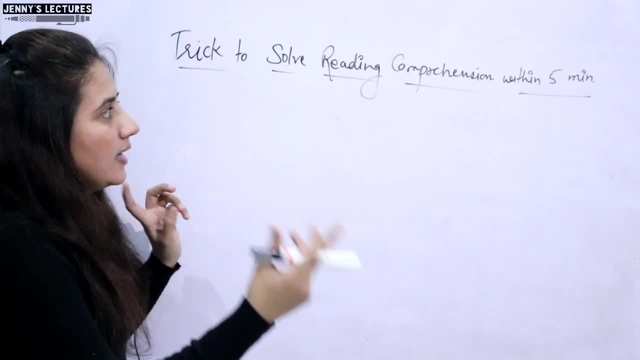 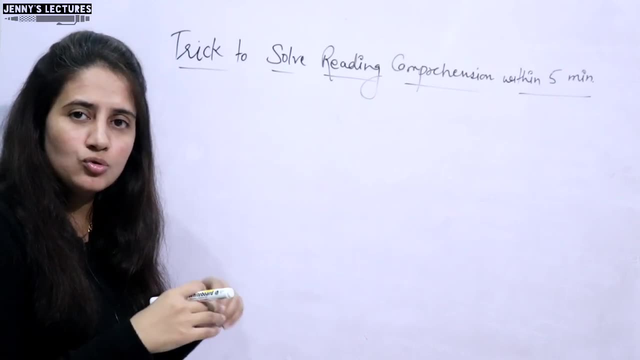 and you have less time. So rather than solving at the beginning, at the end, what you can do in the first go, you can solve the question- easy questions, right Within one minute. you can solve those questions and then you can come to reading comprehension. 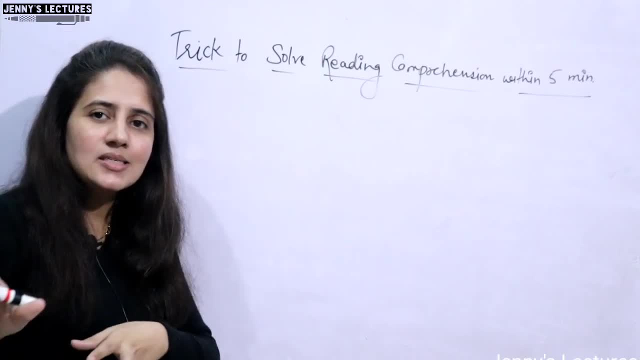 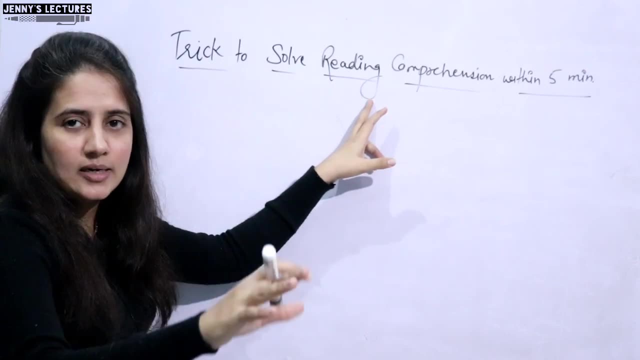 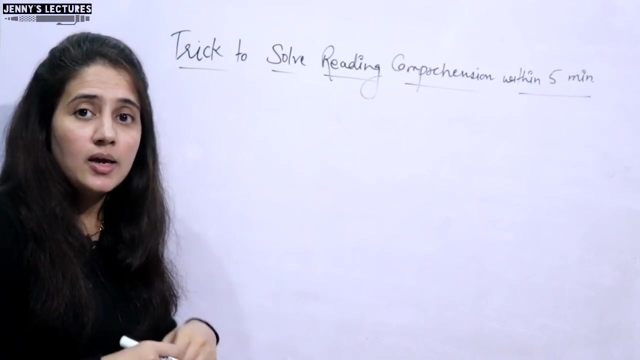 if you are good at this thing, But suppose if you haven't practiced anything, if you are very afraid of this thing, then definitely you should leave it at the for the end, I guess. in my opinion it is one of the easiest unit for you: paper one and scoring as well. 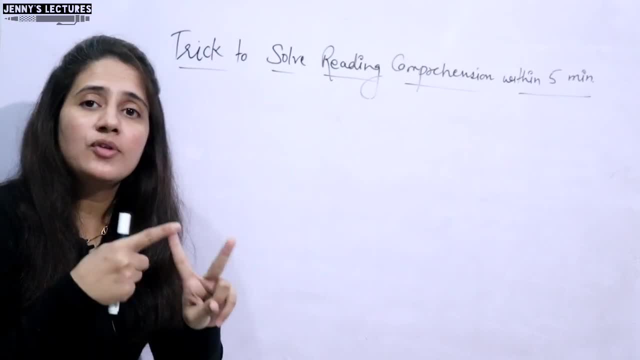 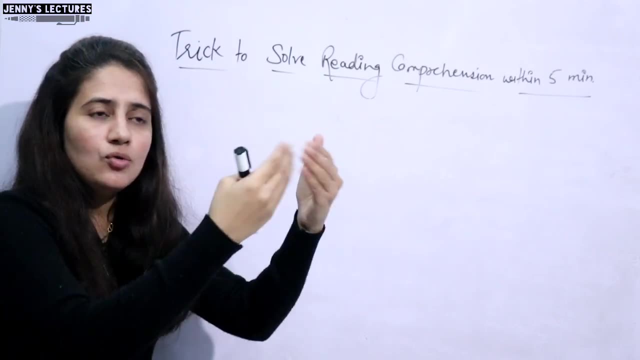 because it is not that tough. out of five questions, two questions would be very easy. Two questions you can say direct questions are there, You can just read the question and directly you will find out the answer within three, four or five lines of first three. 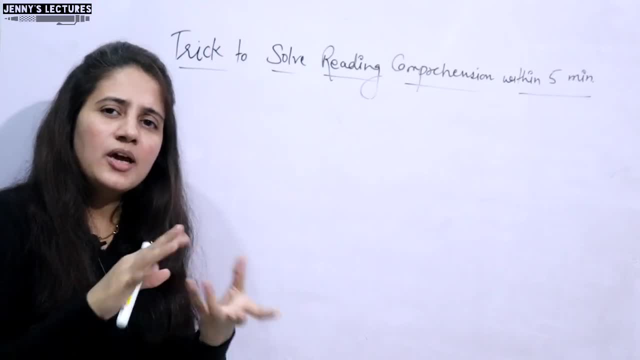 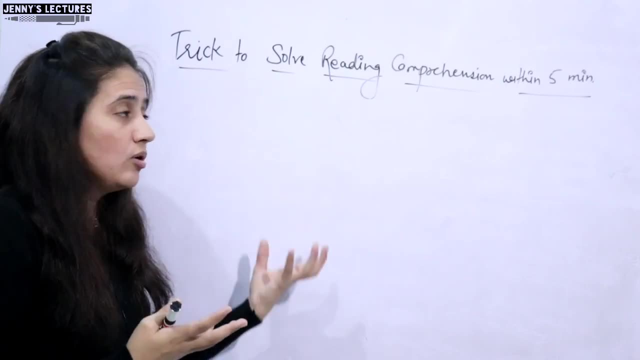 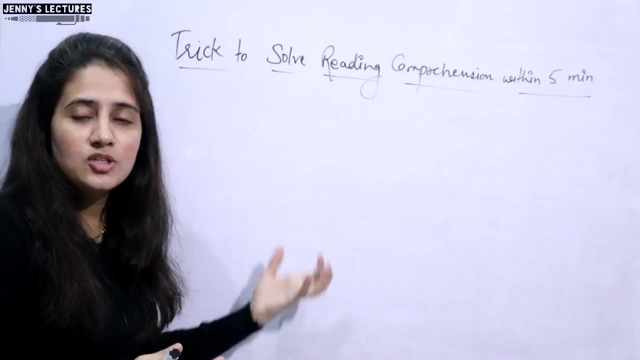 four or five lines of that passage. Two questions would be average type of question and one question is difficult question or you can say indirect question. they'll ask what is the moral of this given passage. or maybe they can ask the title of this passage or what the author trying to say in this passage for answering of. for to answer that. 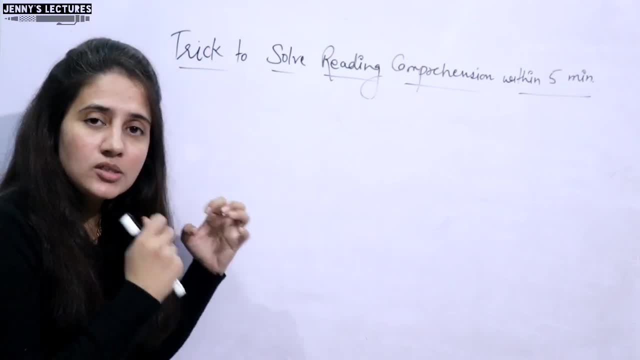 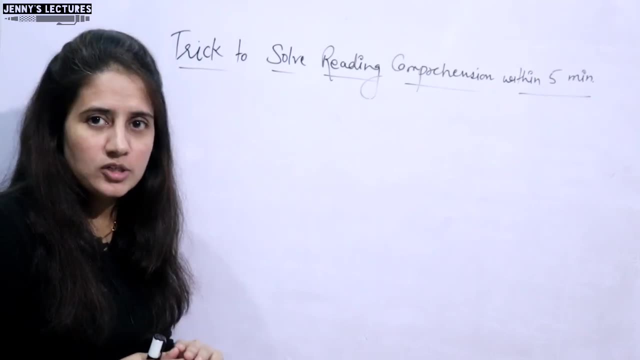 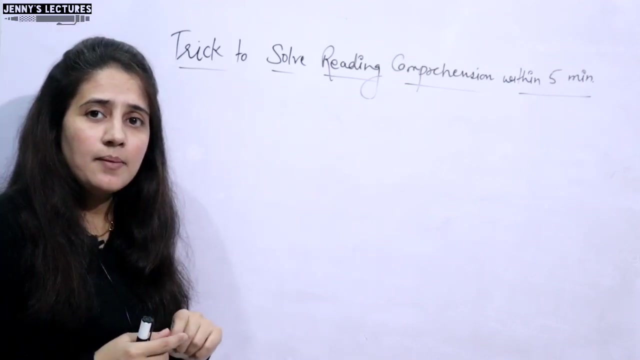 question. you have to read that passage thoroughly. you have to understand the gist of that passage. maybe that would be difficult for you, but you can easily attempt three to four questions if you, if you follow a smart approach. so how to solve reading comprehension, see in net exam. 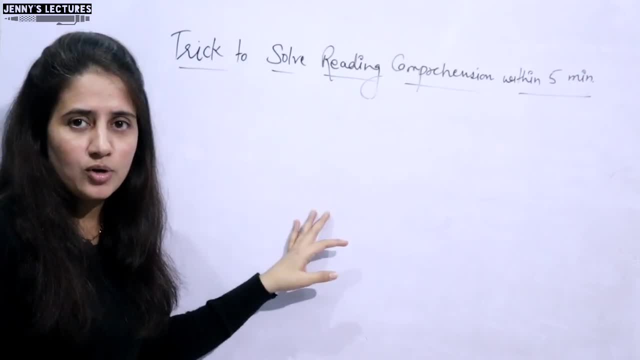 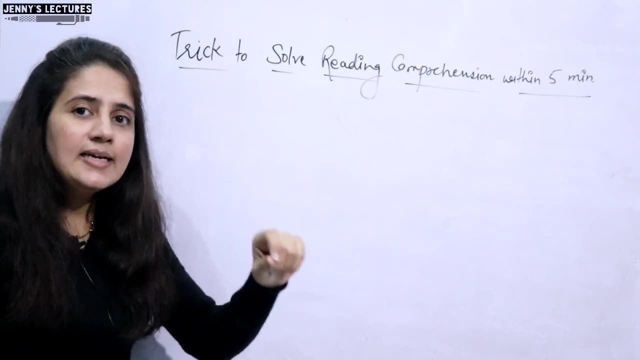 you don't have much time to read the passage, then read the question and all. don't follow this approach that first read the passage, then come to question what you have to do directly read questions. so don't read the passage, first read the question. suppose you are reading first. 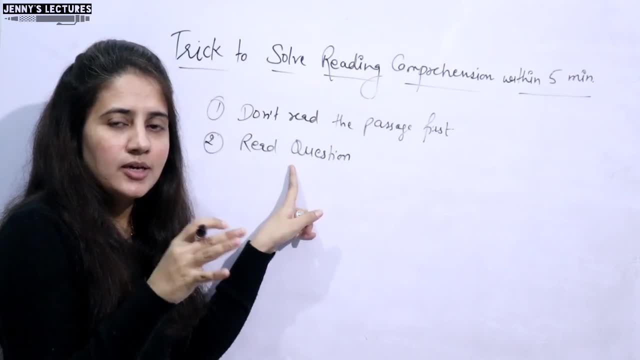 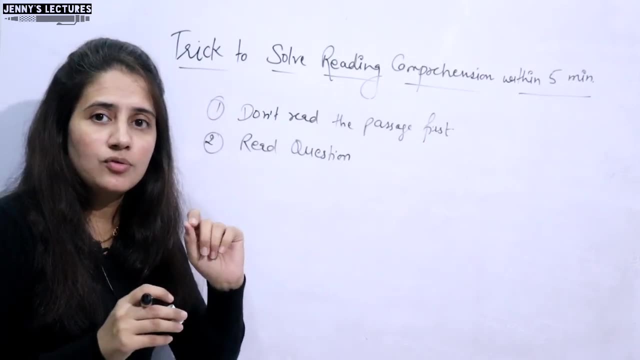 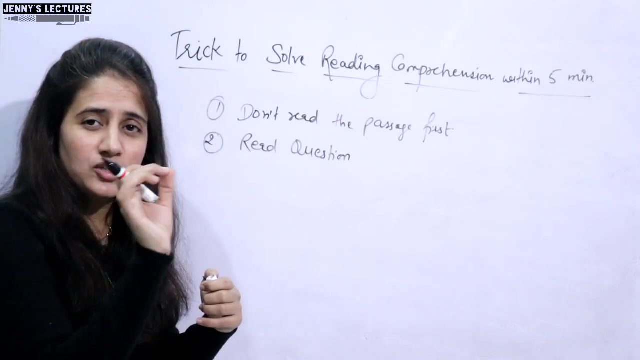 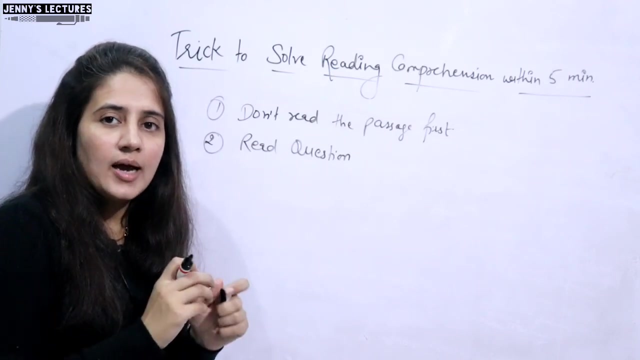 question right, carefully, because sometimes in question you have to take care of these kind of words like not, not true, or only these kind of tricky questions they can ask right and try to write down the you know special or you know special kind of words or keywords you can say or lines you can say from that question and just watch out the options. 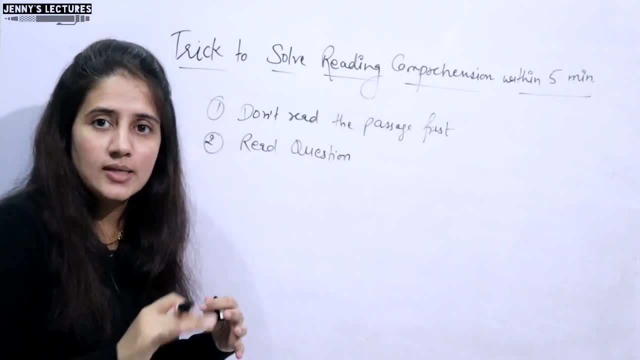 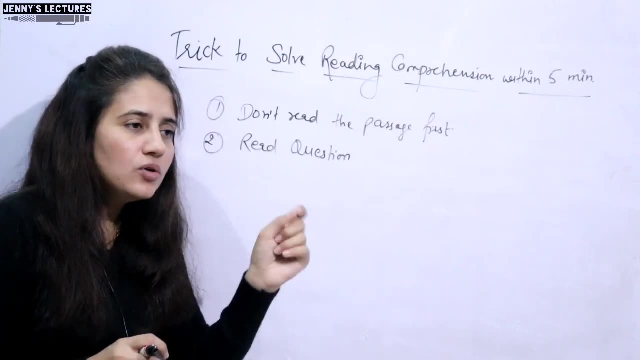 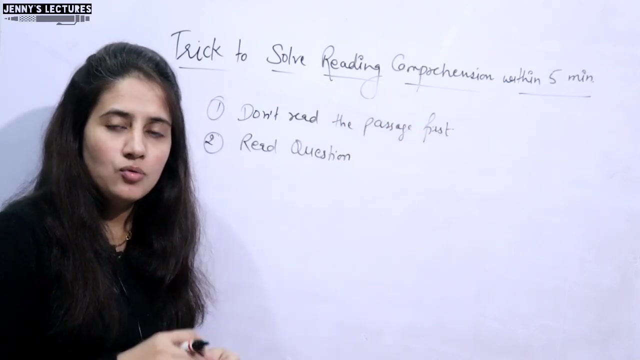 given. you don't have to memorize the question and the answers given. you just have to go through those uh questions and the options to highlight some main keywords given in question and answer right after that, directly go to the passage and try to find out those keywords or those lines or maybe those. 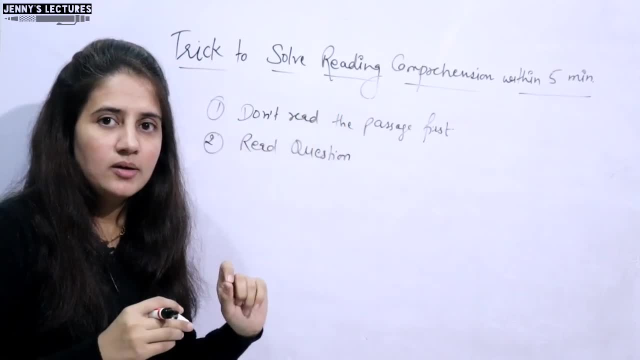 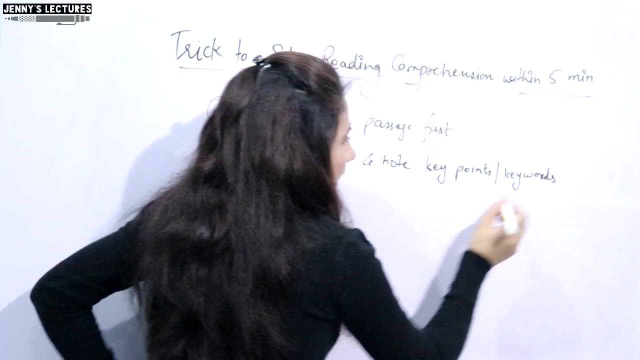 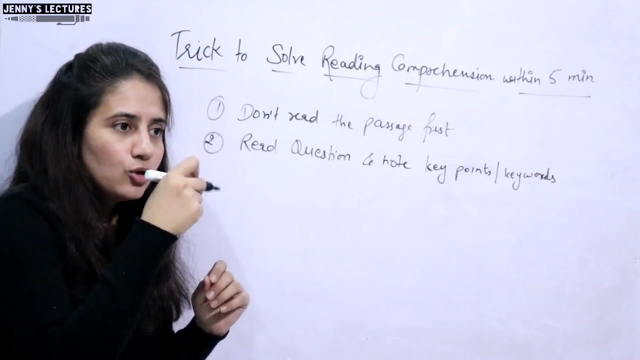 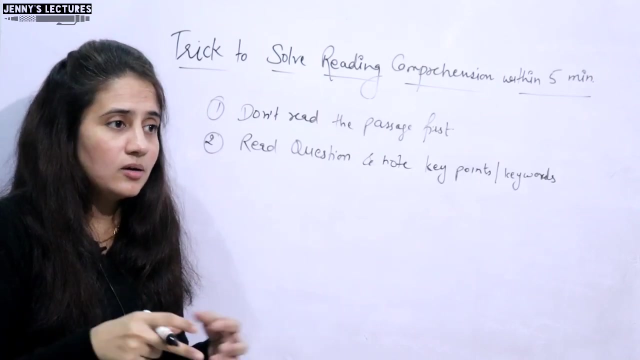 numbers in that passage? right, i think for first two question you can easily find out the answer within first four, five lines of that passage and while reading, you have to read that passage with, with full concentration. it's not like that you are reading that comprehension and after reading three or four lines you are, you know, lost somewhere. and 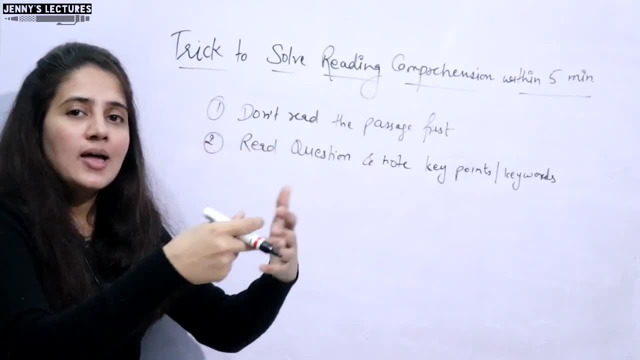 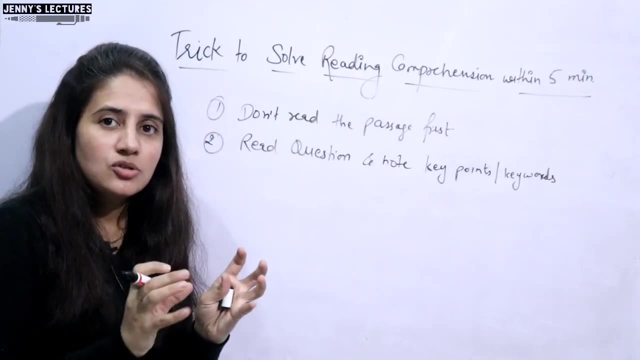 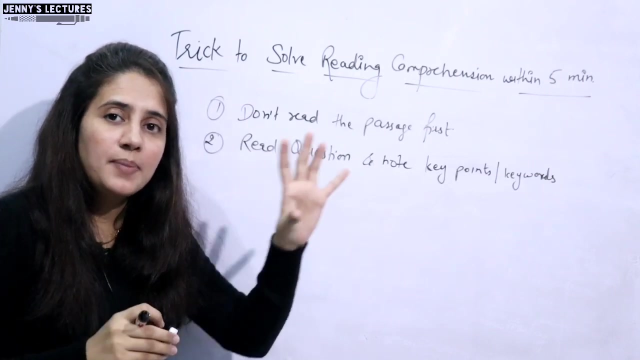 you haven't get anything from those lines. you have to visit that passage again. so this is what wastage of time. with full concentration, read that passage at the first time. only that you will get what is there in those lines. maybe you don't have to memorize the passage. also, don't have 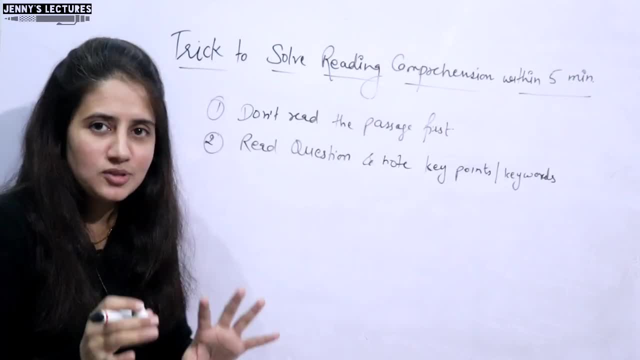 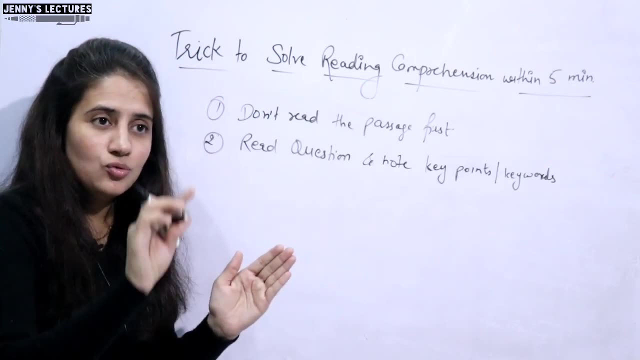 to memorize the passage. you don't have to memorize the question or the options given, right, but you have to read that passage with full concentration, with attentive mind, like in first go. you can find out answer of the question, right, if see, if you will read question first and if you. 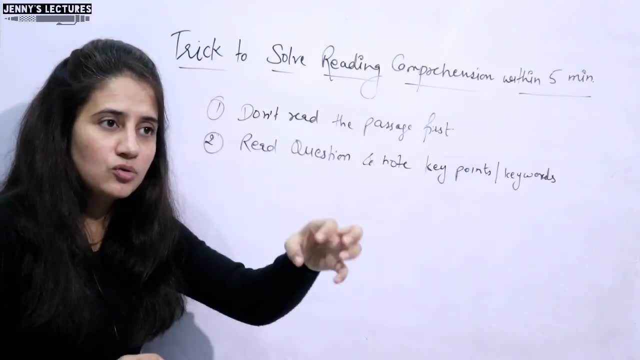 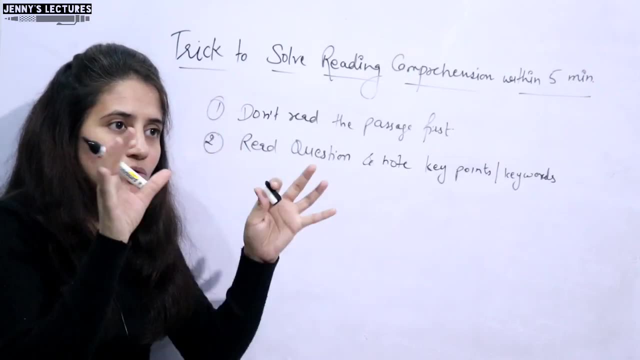 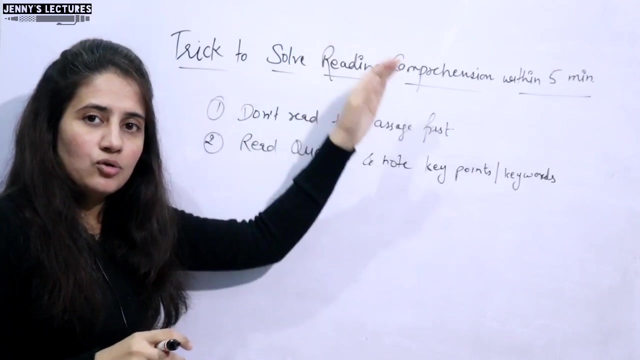 will find out some keywords or some key points from that question or from that options given. then when you are reading that passage, your mind is what, trying to locate those keywords, and at that time it would be more attentive rather than without reading the question and you are reading the passage. at that time you will not get anything from that passage, i'm damn sure. 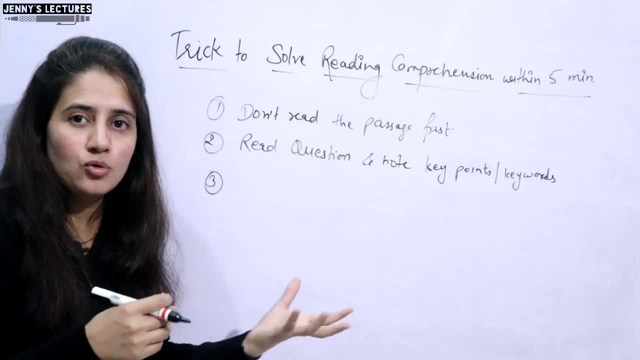 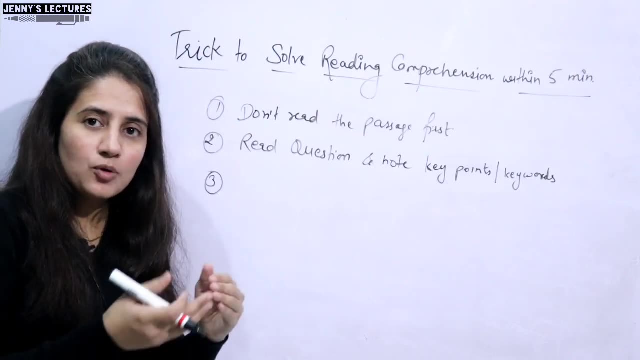 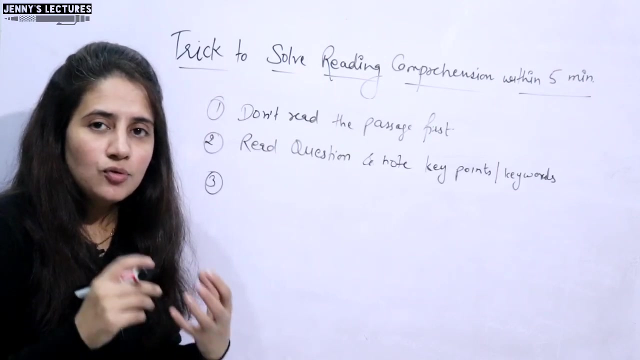 and sometimes maybe you find that keyword or that key point of that question in one line of that passage, but still it is not the answer of that question. maybe the answer is within surrounding two to three lines. you have to read more lines to get the answer. so you have to focus. you have. 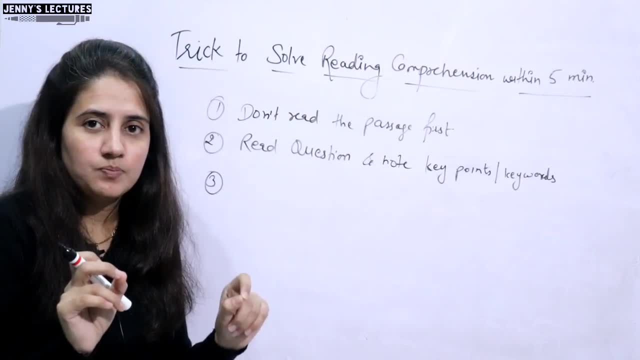 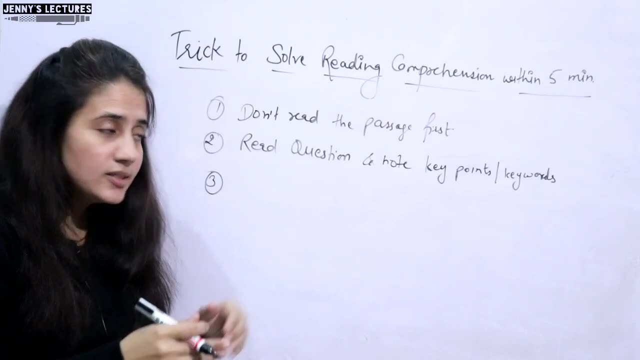 to read question very carefully. that is very important- and then try to find out the answer. and next, i have already told you, do not try to memorize the passage while reading. see, for first question you have done this thing. for second question also, you have to do same thing: read. 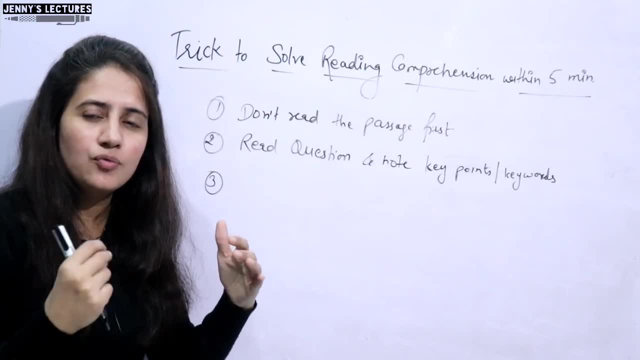 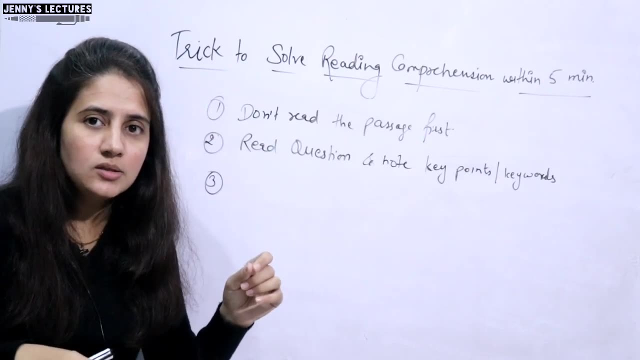 question. read options given within just you know few seconds. try to find out, try to you know, write down those keywords or main points of that question and answers and then directly jump to that passage. try to find out those keywords and try to find out the answer of that. 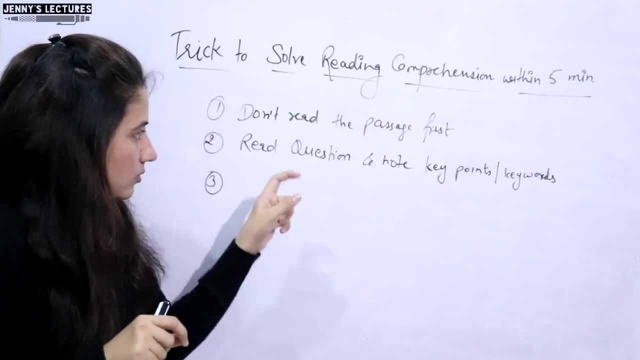 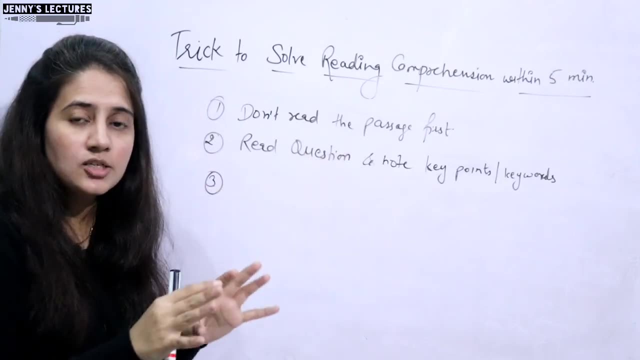 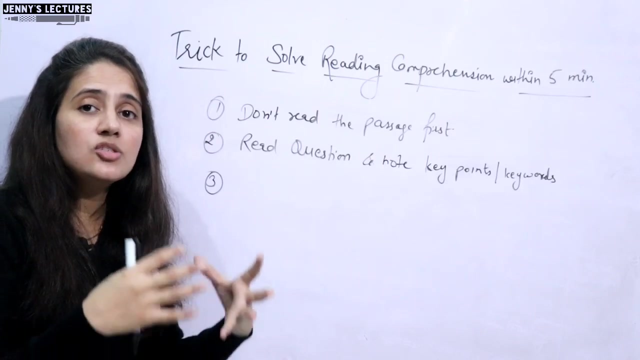 question right now, while reading that passage for these questions. it's not like that you just find out the answer of these question. that's it you have to understand. try to understand the passage. try to understand the gist of the passage, what the author is trying to say at that time. only because maybe fifth question is like this indirect question based. 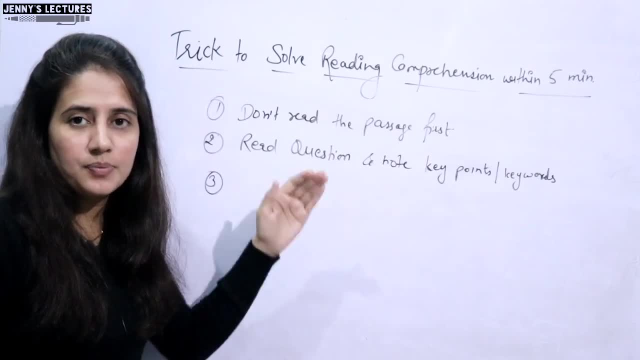 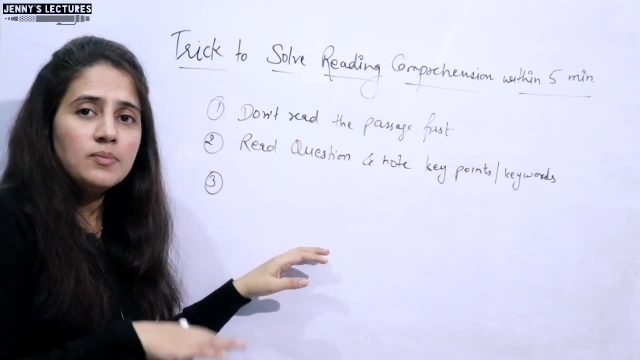 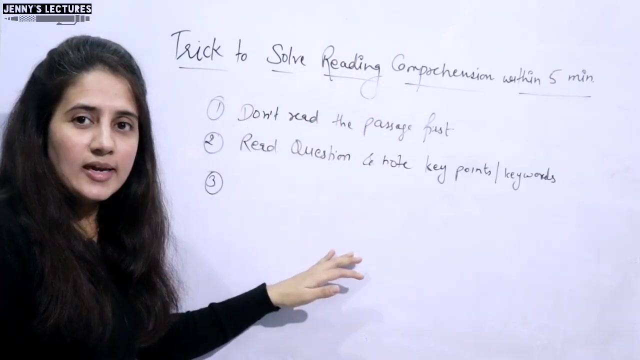 on your understanding. maybe they are asking the tone of that passage, what is the title, or maybe what is the moral or something like this, right, so it's not like that. it shouldn't be like that. for fifth question: you, you need to read the passage. read that passage again. no, while reading that passage for answering. 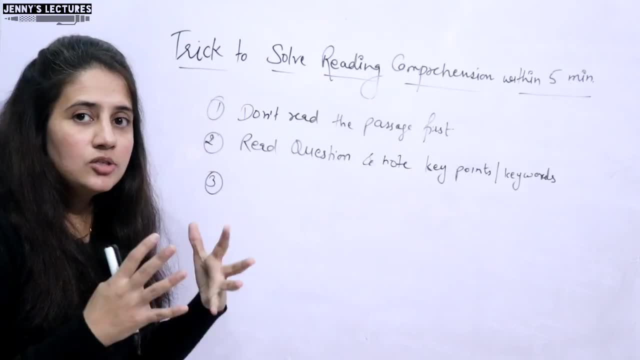 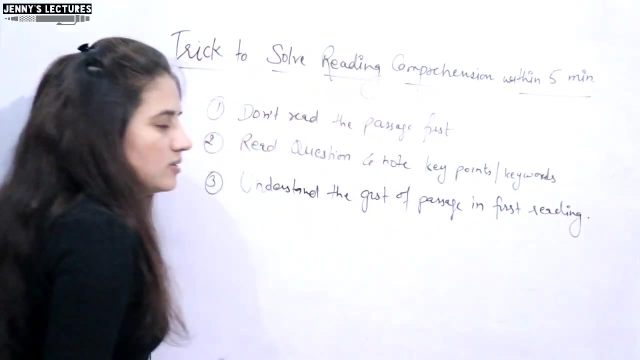 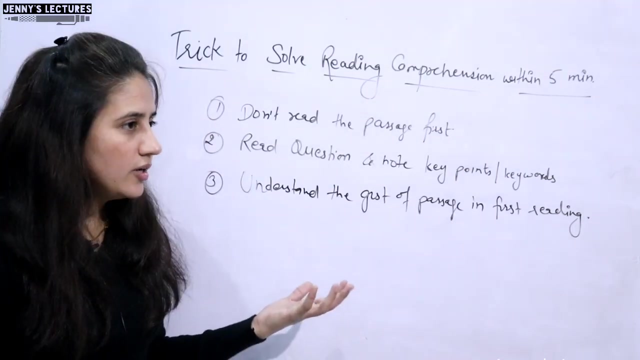 the questions: first, second, third or fourth question. just try to understand. try to understand what the author is trying to say. so try to understand the gist of that passage in first reading only. and next step is: if you got stuck somewhere in the passage, suppose, if you are not getting answer. 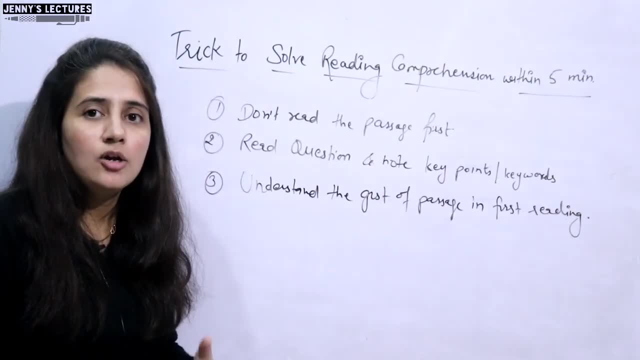 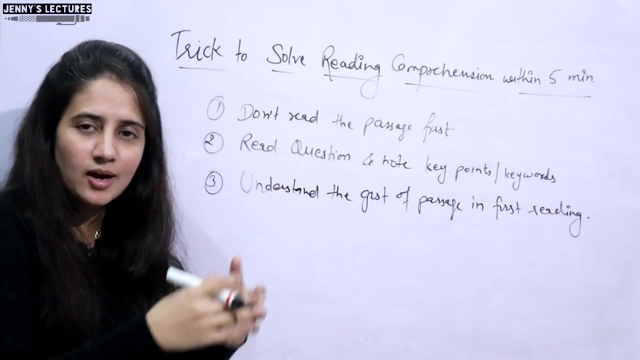 meaning of any word or any line. if you are not getting any line, do not stuck at that line, right? it's okay if you are not able to understand that line. if you are not able to understand that word, skip it and read next line, right, do not stuck somewhere, do not try to. 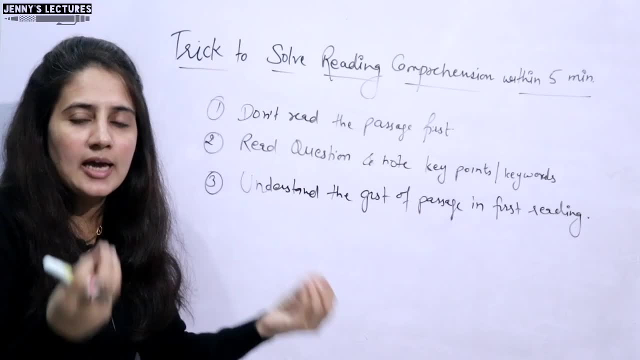 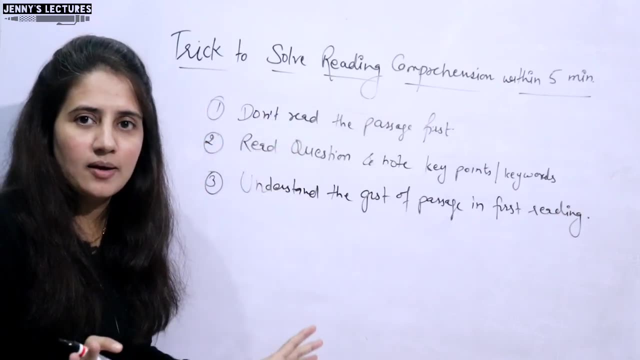 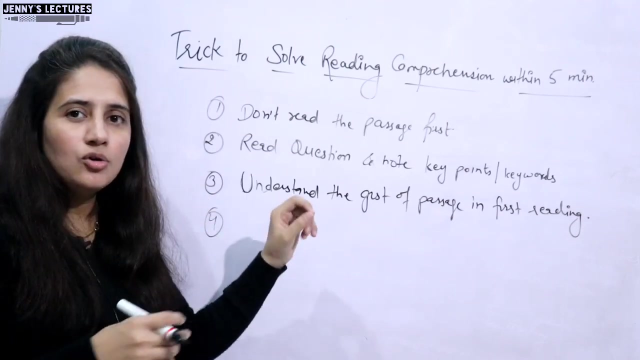 understand the meaning of each and every word given and each and every line given in the passage. right, it is not important, you have to just try to understand the gist of that passage. main idea right next is: do not waste much time in finding answers like: suppose in first reading you're not. 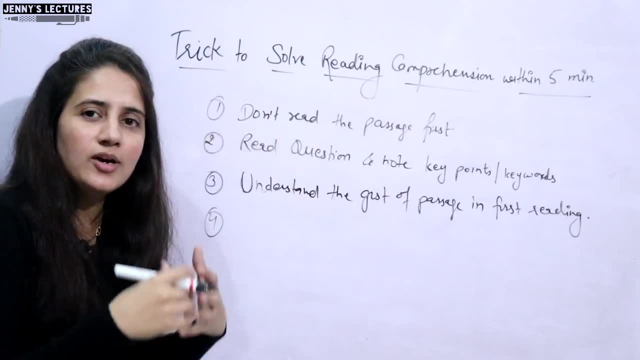 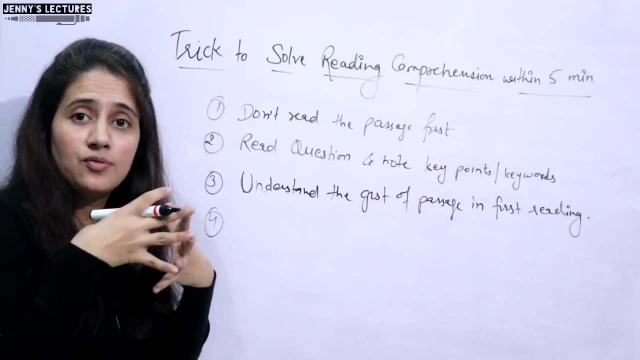 getting the answer. suppose you are good at reading. second time also, you have read quickly and but still you are not getting the answer of that question. leave that question. do not stuck at that question, like i will find out answer of this question. definitely. if you do so, then definitely.